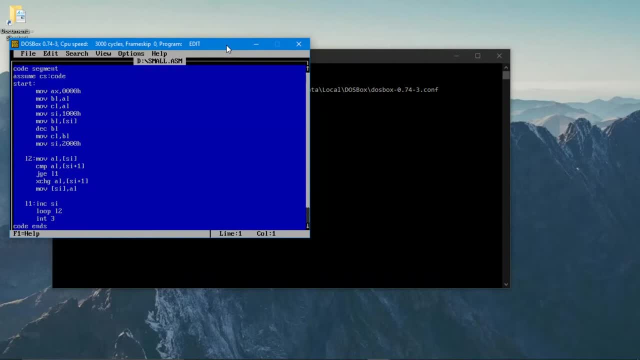 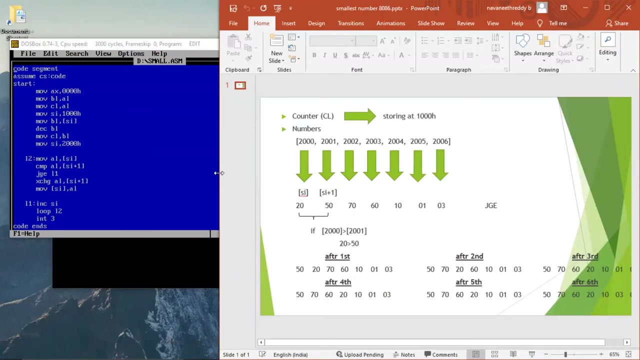 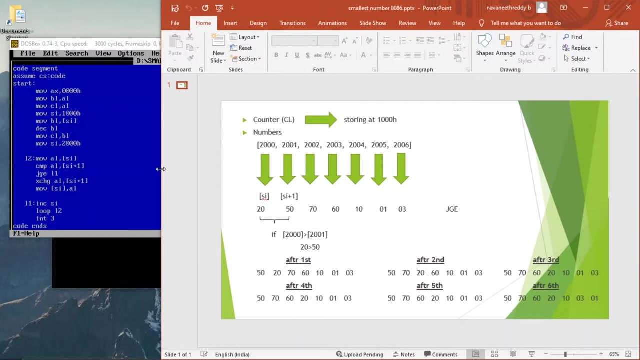 Now, without directly entering into program, I just want to give a brief overview What is going in this program. So let me open my PowerPoint. you a sec. Okay, I think it's visible. Let me drag over here, Yeah, Okay. so the number set we are going to give our program in this particular video is: 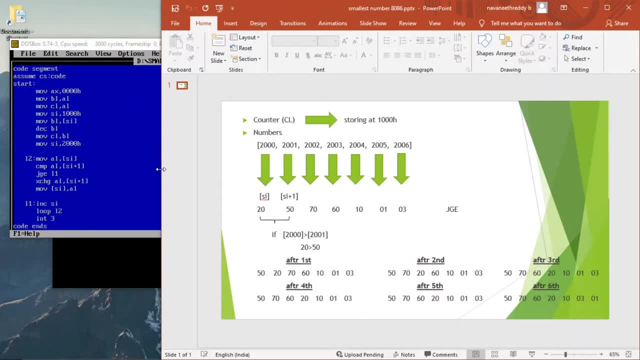 this set starting from location 2000 to 2006, that is, a 2000 location 20 and a 2001 location 50 and 2002, 70, 2003, 60 and, up to 2006, 3. so the number set we are going to give to our program in this particular video are: 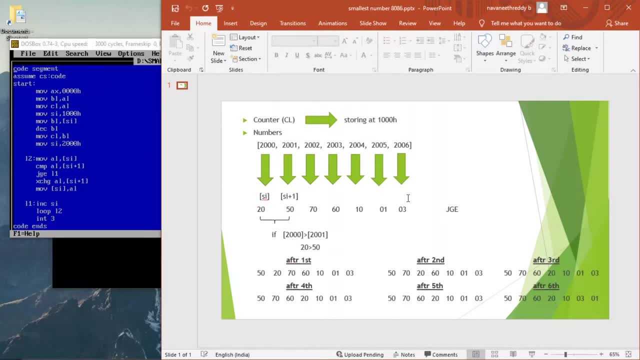 20, 50, 70, 60, 10, 1 and 3. so our program should give the output 0, 1. that is the. that is what the least from this set right. So if we, our program give 0, 1 as output, our program is working fine. 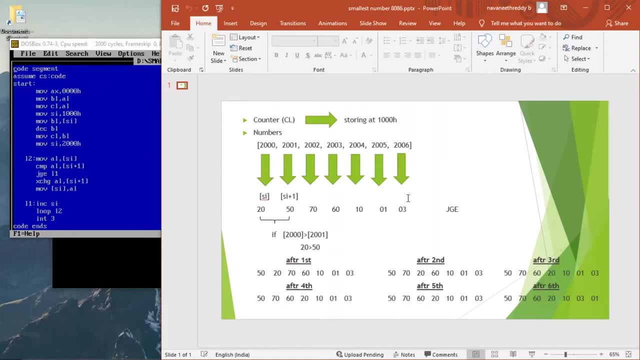 so How our program is going to figure out the least, that is 0, 1 in our case, We are going to see in this video. so the logic over here is You have to be familiar with this mnemonic code that is JWE jump greater than or equal to. 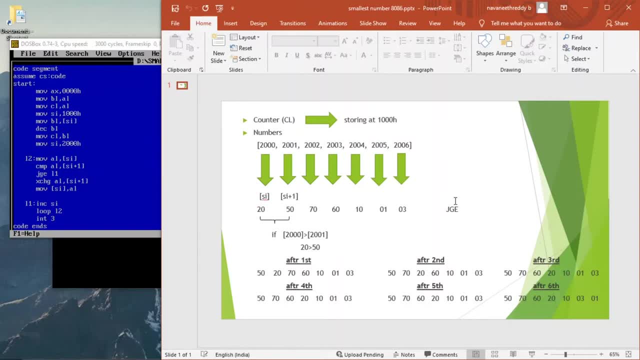 Our total video will revolve around this command. actually I mean that mnemonic code. so the logic we are going to use here is Now: just concentrate on these first two numbers of Go, pair by pair, that is, in first iteration 20 and 50, the next iteration 50, 70, the next iteration 70, 60, like that. 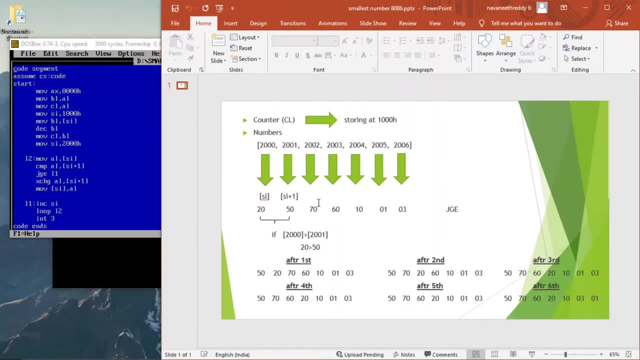 Just navigate to pair by pair. So in the first iteration we are in the first iteration, So we are taking this first two pairs, that is, 20, which is at SI location, and 50, which is at SI plus one location. so we will compare these two, 20 and 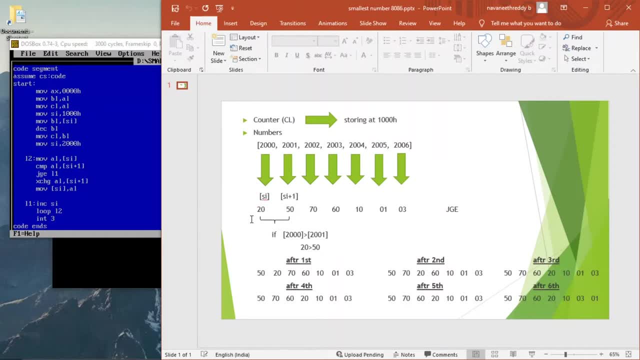 50. that is the first pair. and If the first number is greater than second number, Will jump. that is, jump greater than equal right. So if first number is greater than the second number, jump to some other location and do some stuff over there. But if first number is not greater than second number or smaller, 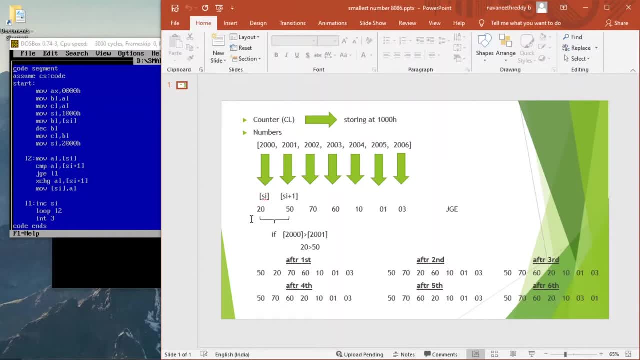 Just exchange the two locations, that is see, in our case here, 20 is not greater than 50, right, So that condition fails, that is, jump greater than or equal to. so we can't jump and we are not going to jump anymore to any location. 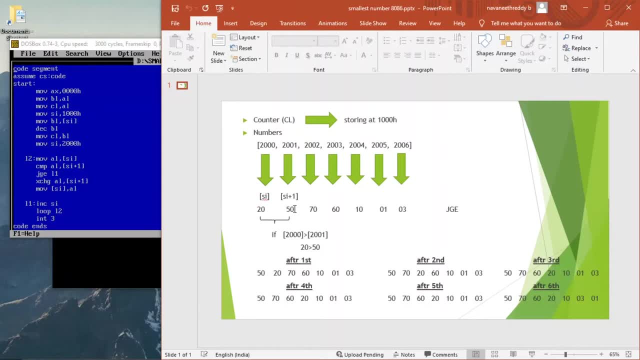 So what we will do is, instead of jumping, will just swap these two numbers. That is, 20 will come to 2001- location from 2000- and 50 will come to 2000- location from 2001. Just swap these two numbers, That's it. 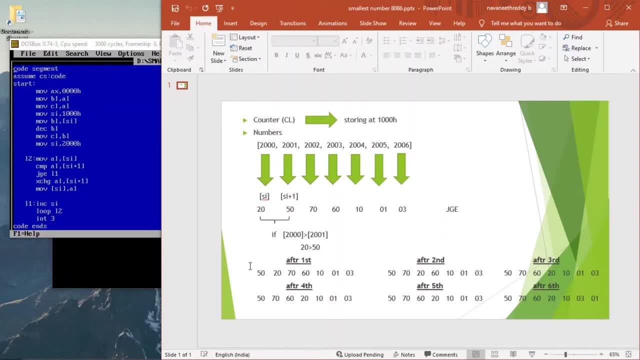 So after first iteration, our number set will look like this: 50, 20, 70, 60, 10, 1 and 3- that is, just 20- came to second place and 50 gone to first place. Now in the same way. now go to the next pair. What is the next pair? 20 and 70 right now in the 50 is completed. 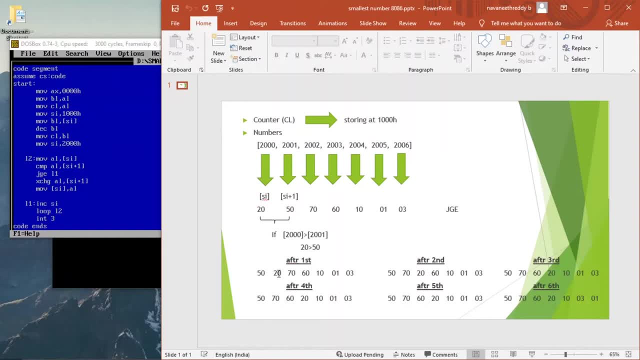 Now in the same way. now go to the next pair. What is the next pair? 20 and 70. right now in the 50 is completed Left, leave it alone. Now just go to second pair, 20 and 70. Now compare these two whether first number is greater than 70. 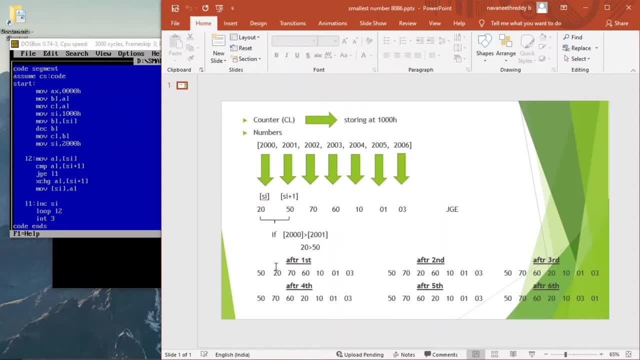 I mean second number or not. if greater, go to some other location. That is, with the help of this JGE, jump greater than or equal to some other location and do some stuff. if not greater, That is, if first number is not greater than second number, Just exchange the two locations and in our case here 20 and 70. 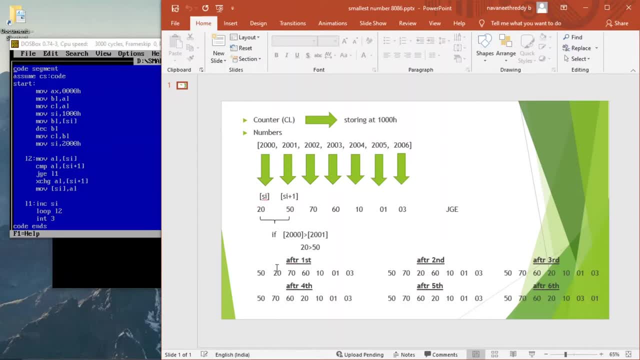 20 is greater than 70.. No, so we are not going to jump anywhere. instead, We will simply exchange These two locations. that is, 70 will come to 20 place and 20 will come to 70 place. So after second iteration, our number set will look something like this: 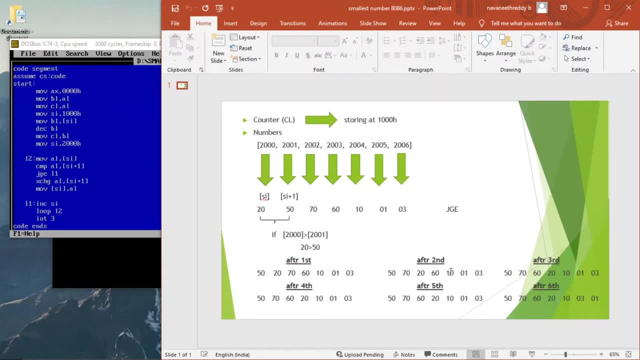 50, 70, 20, 60, 10, 1 and 3. so like this it goes on. But up to how many iterations? it should go right. We should have a number right and that number is n minus 1, that is, if n is the number of. 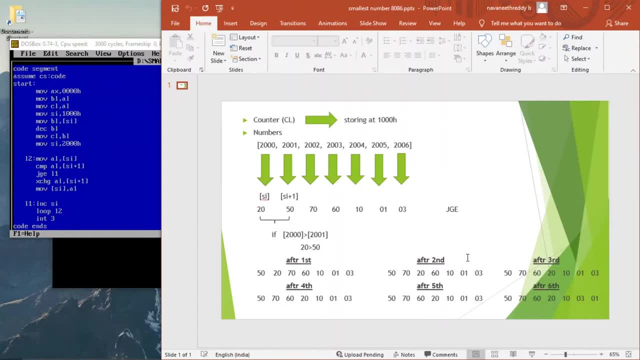 Numbers in our set. that is here. How many numbers are there in our set? 20, 50, 70, 60, 10, 1 and 3, right, that is 7. So if there are n numbers in our set, It will take n minus 1 iterations. 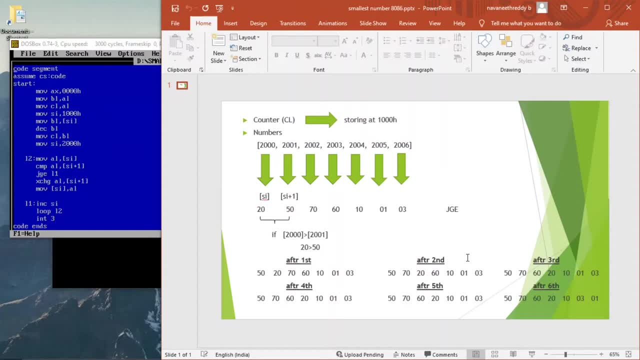 So that n minus 1 number. where we should store? we should store in the counter. that is CL register. So that's why we will use CL register in our program. So what is the use of CL register means? In order to store the counter value, that is. 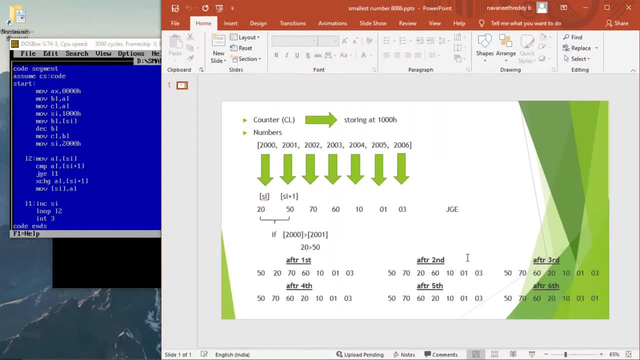 Till it becomes 0. we will loop these instructions. See after first iteration will Do this. that mean I will check this condition. and after second iteration also, we are checking the same condition. For third iteration. we are checking the same condition, So instead of writing the code repeated, we will use the loop over here. 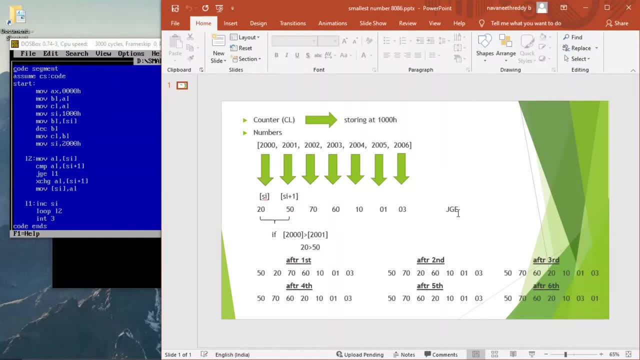 I mean loop mnemonic code. what that loop mnemonic code will do is It will jump to the location provider over there till CL becomes 0. so In our case now CL is 6, So it takes 6 iterations in this case, as we are giving 7 numbers. 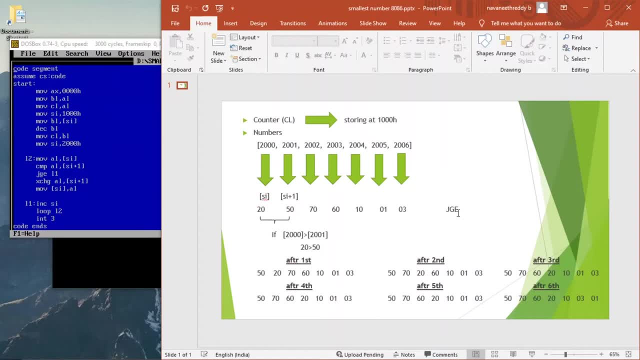 CL value will be 6 and until it becomes 0, that is, it will execute the same set of code 6 times in our case. So, like this, just take next two pairs, next two pairs And just go on. and if your first number is greater than second number, 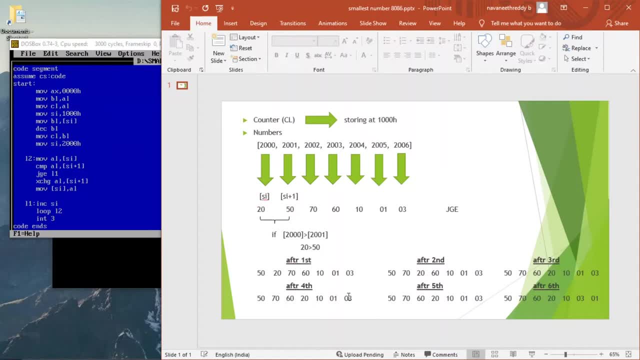 Just jump to some other location and do some other stuff. if not greater, just swap the two locations. See now, you can see over here, 10 and 1. right now 10 is greater than 1. So what we have to do, we have to jump To some other location. we should not exchange here. 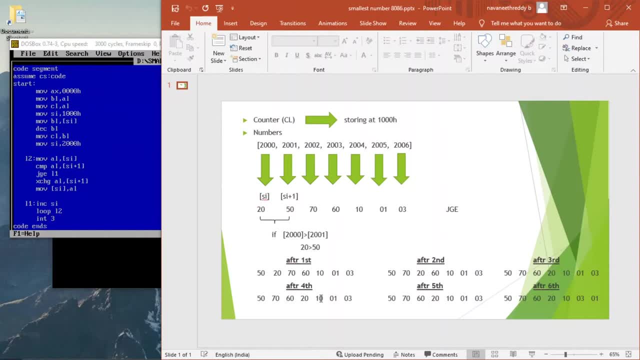 See, because first number is greater, that it is true. So we have to jump to another location and do some other stuff. So what we'll do that there nothing will do. just we will keep the numbers as is and we will go to the next one, That is 193. so after the fourth iteration 10 will be in the same place. 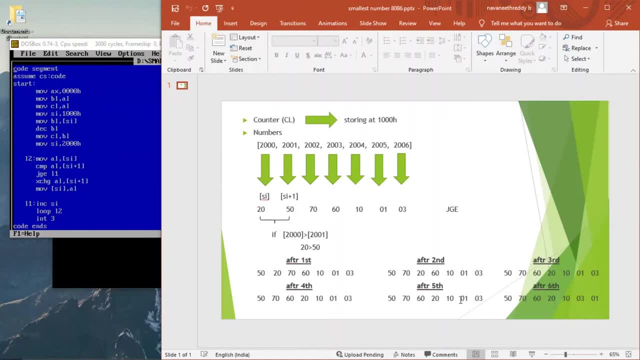 Now we will go to the next two numbers and we will again check whether this first number is greater than Second number or not. if it is greater, we will jump to some other location and we'll do some stuff over there, and the Stuff we'll do is nothing, just keep the number in its place. 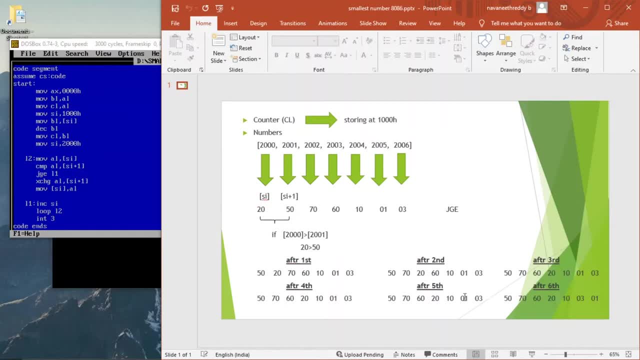 And if it is less we'll swap the location. here one is less than 3, right? so we are swapping the location. So 1 will go to the last place and 3 will come to here. So we will continue the same iteration. still, the smallest number is 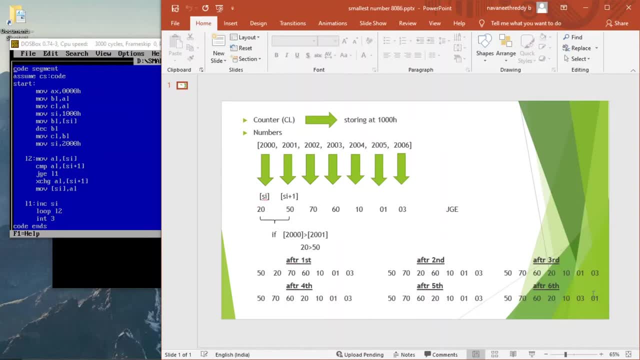 achieved in the last address. So you have to one thing have to remember: over here is our answer that the least number will be available- available in the last address, that is, 2006 in our program. so I think you got a brief idea on how to figure out the least number. now we will see the program. ok, the first three. 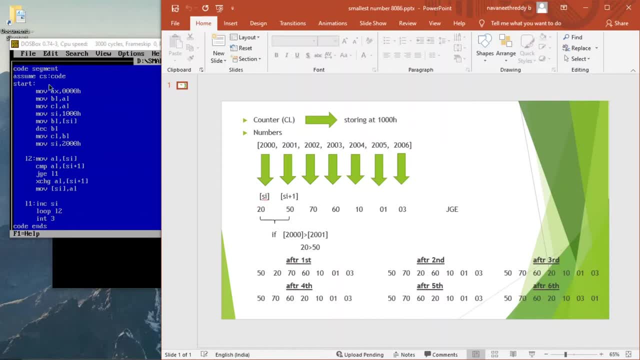 lines are same as usual and we are not using data segment in this program. so just write code segment and assume cs code and start. those are the boiler plate of our code. you know, and the first thing we are in any program, the first set of the program will be clearing. 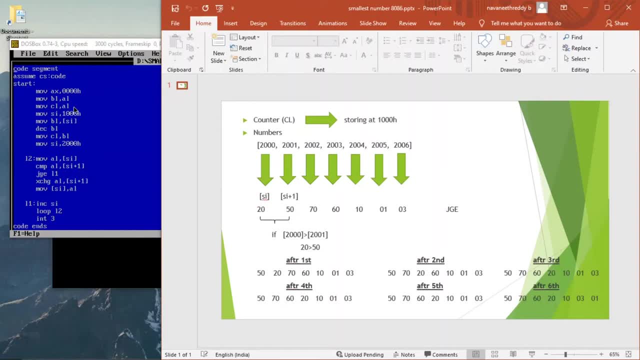 the registers, what we are going to use here. we are going to use al, bl and cl. ok, so with this move x, move ax, comma 0 0 0 0 h, we are clearing the al ax register. that is, indirectly, we are clearing ah and al. right, so al is cleared and ah is also cleared with this instruction. 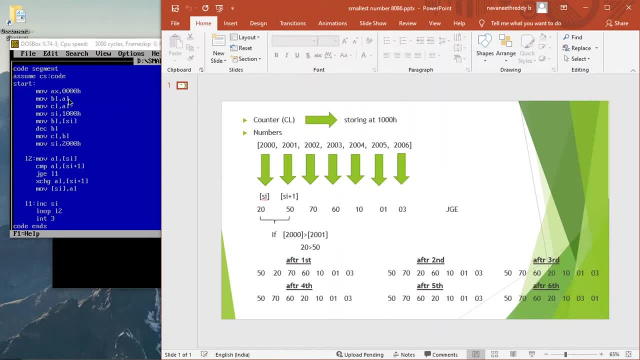 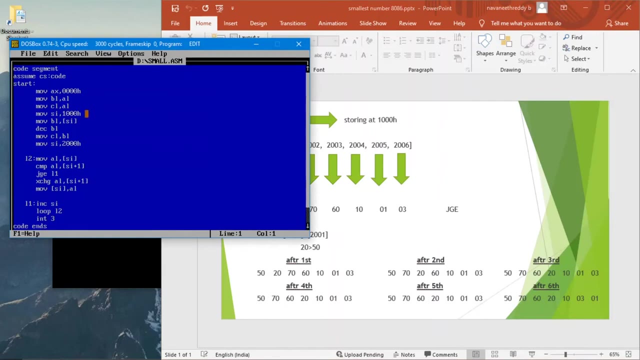 now we are moving that cleared value of al to bl, so that bl is clear, and in this instruction we are clearing the cl as well by moving the al value into cl. ok, that's finished now. and with this instruction, that is, move si comma 1000 h, we are making si point 2000 h and with 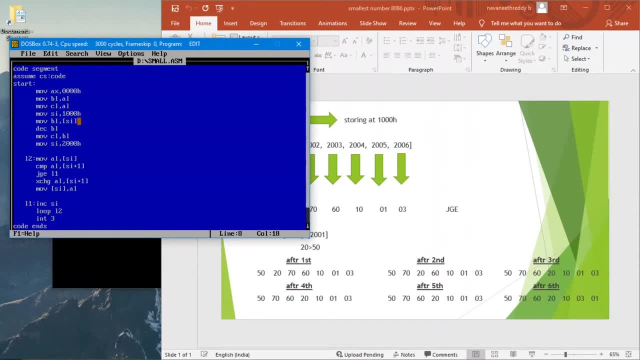 this instruction, that is, move as bl, comma, location of si. we are transferring the content at location 1000 to bl and the next thing we are doing here is decrement bl. that is, if bl value is 5, decrement bl does is it just decreases by 1. that is after this instruction. 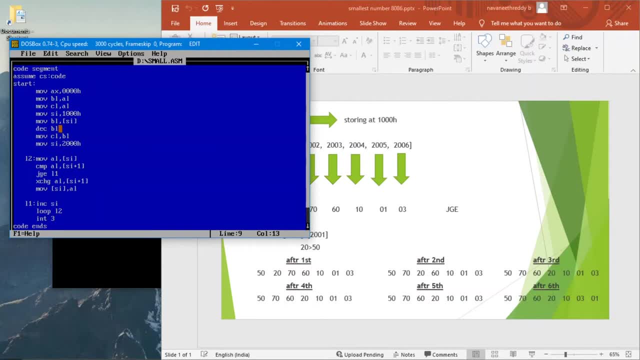 bl value will be 4 and if you give bl as 7 after this instruction, it's value will be 6. that's it now we are moving the decremented value to cl over 7. that is it. now we are moving the decremented value to cl over 7. now we are moving the decremented value to cl over. 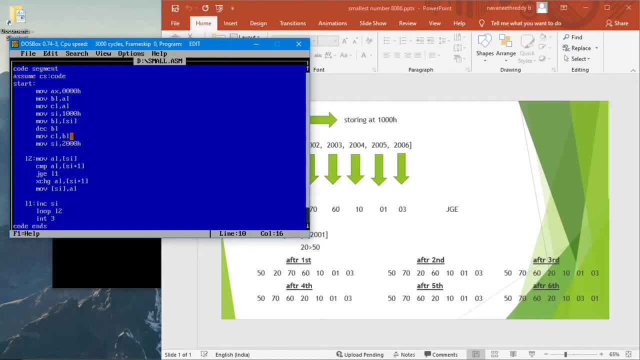 here with this instruction, that is, move cl, comma bl, why we are decrementing and giving the value. i said: right, if there are n numbers, n minus one, iterations are required. so, and that number should be stored in cl, right. so here, first of all, we are taking that number into bl and, as we require, only. 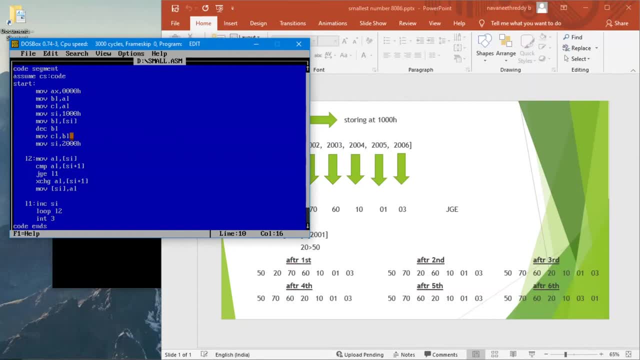 n minus one iterations. we are decrementing it by one and then we are moving that decremented value to cl. that's it. and now again we are pointing to si, to 2000h, so that we can give the input values. so this, i mean this set, is the program where we clear all the registers and we are making use of 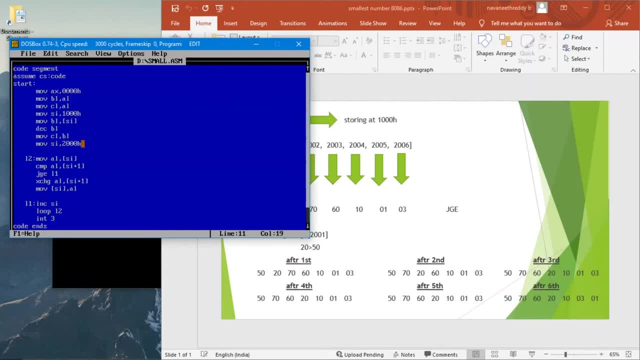 this cl and we are initializing that cl and we are pointing si to 2000h again. now leave this move sl comma 1000h. that is finished. that is just in order to initialize bl and cl. now we are again making si point to 2000h and from that 2000h that is the content available at 2000h. we are moving. 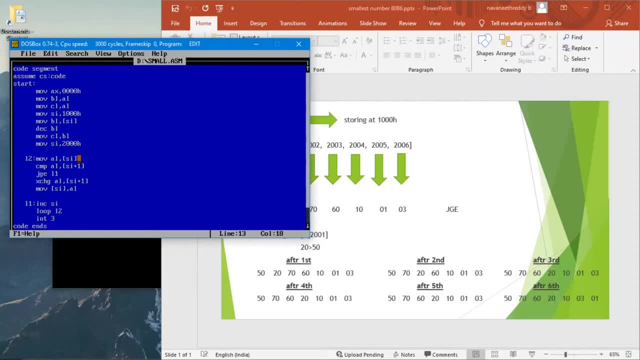 into al with this instruction, that is, move al comma square brackets of si. now here, what is this cmp? compare al comma, si plus one. see, i said we have to compare the two numbers pair by pair, that is, the number at si location and the number at si plus one location. 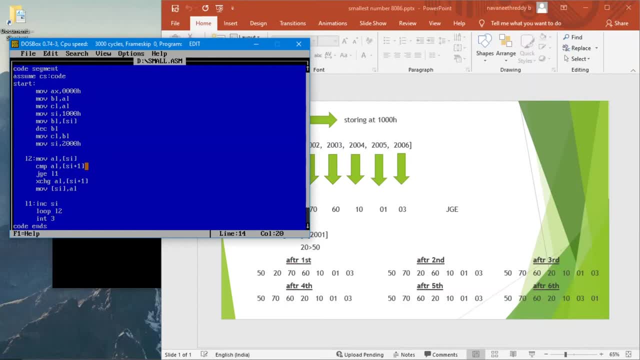 see, that's what we are doing here: compare al comma si plus one. al is nothing but the number at location si, right? so with this instruction, that is, compare al comma si plus one, we are just comparing the two numbers and and in that comparison, if first number is greater than second number, 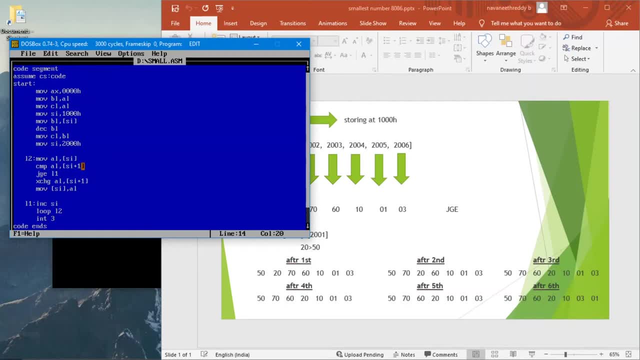 we will execute this command. that is jge, that is jmp greater than or equal to where l1. so here it comes to here. program comes directly to here. if it is not greater, just execute these two commands. what did i say? if it is greater, just go to some other location and do some stuff. if it is not greater, exchange the location of numbers. this is what i said, right? yeah, that is what we are doing over here. if it is not greater, just go to some other location and do some stuff. if it is not greater, exchange the location of numbers. this is what i said, right, yeah, that is what we are doing over here. if it is not greater, just go to some other location and do some stuff. if it is not greater, exchange the location of numbers. this is what i said, right, yeah, that is what we are doing over here. if it is not greater, just go to some other location and do some stuff. if it is not greater, exchange the location of numbers. this is what i said, right? yeah, that is what we are doing over here. if it is not greater, just go to some other location and do some stuff. if, 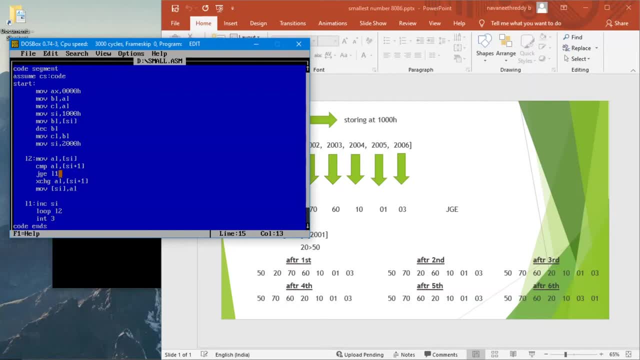 it is jump, greater than or equal. just go to location l1 and what we are doing in the location l1, we are just incrementing the value si by one and we are again comparing. that is, i said you start comparison by first pair and then go to the second pair. so in order to go to second pair, 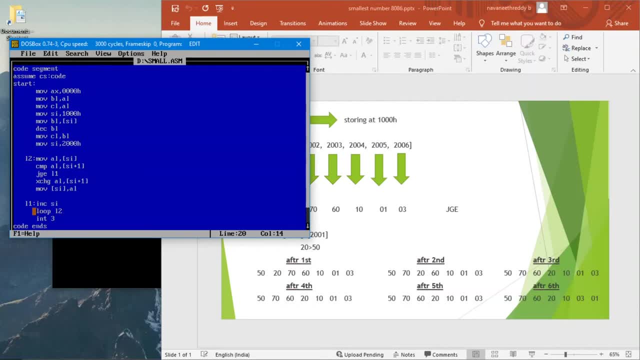 we are using this variable. i mean not the variable but the mnemonic code loop. now again where this loop go to this: again we will move the content of si to the al, and again we'll compare al, comma, si plus one, and again we will check the instruction jge. 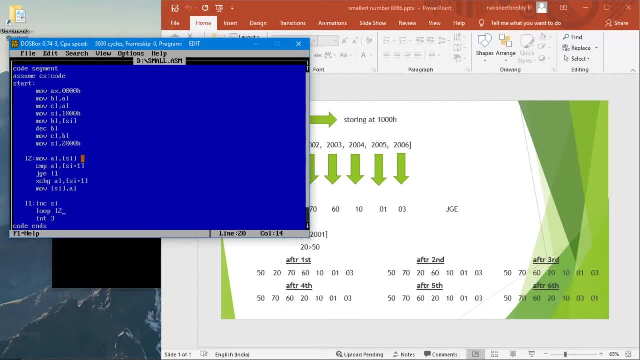 and again. if a first number is greater than second number, again we will come to here and again we'll go to this loop, and if it is not greater, we will just exchange the two locations and then we will check again. the same situation will continue, and until cl becomes zero, only this, this program, i mean this set of l2, will execute. 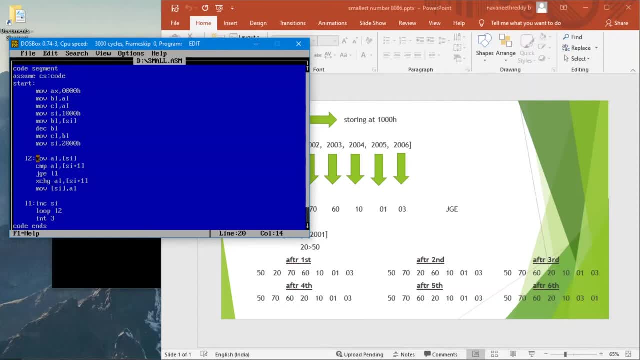 once. if cl becomes zero, it stops execution and the program ends, that is, with the help of int3, and code ends. i think you got an idea. uh, if you don't have a perfect understanding or nothing will happen, just repeat the video once more, or if you have any kind of dots, feel free to contact me. 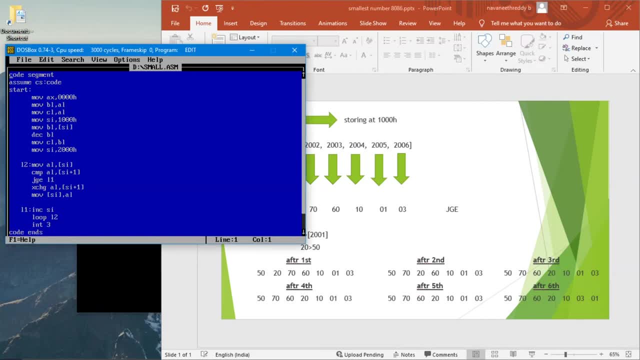 yeah, now let us execute our program and in my case i actually opened already saved file, so no need of seeing for me. but in your case just go on to this file and click over here, save as and just give a name, but make it relevant to the program. but the extension should be dot asm. okay, in my case i'll directly exit from here. 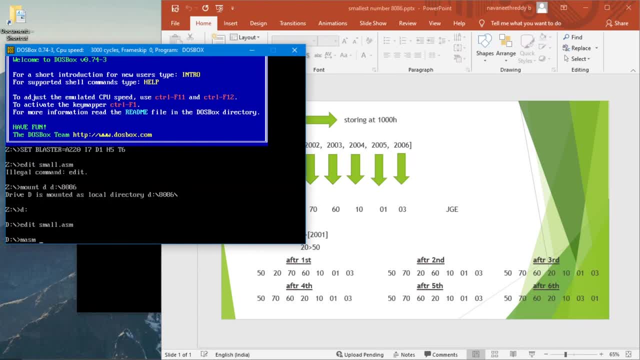 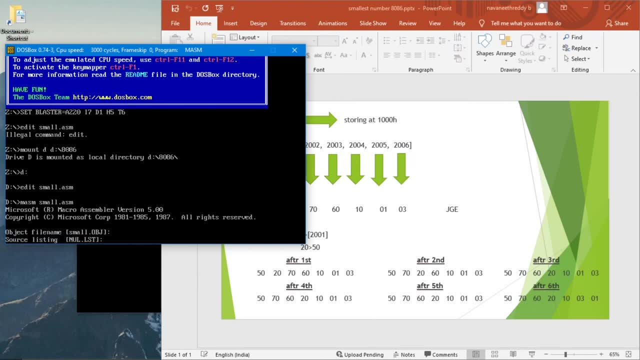 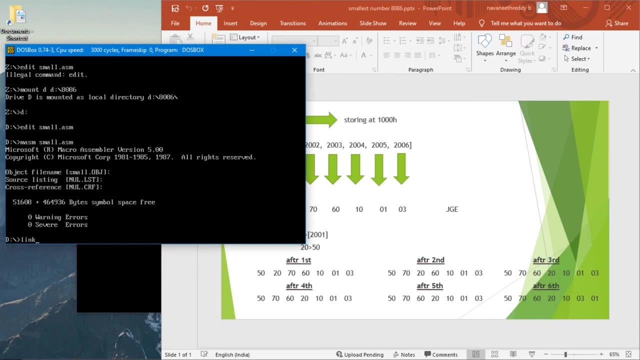 and the first command we have to give in order to execute our program is massum and the file name dot asm. right and click four times enter and our program is generating zero errors. that's a very good sign, actually. and the next command is a link and program name, dot this time. 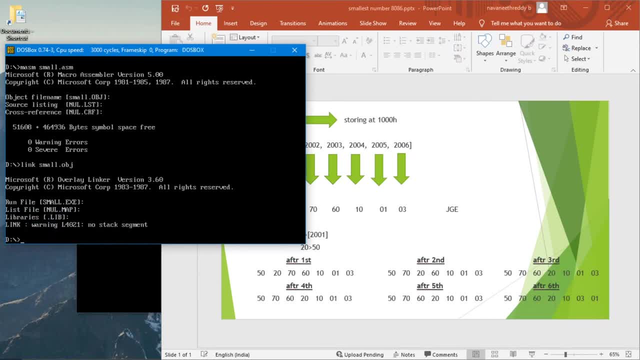 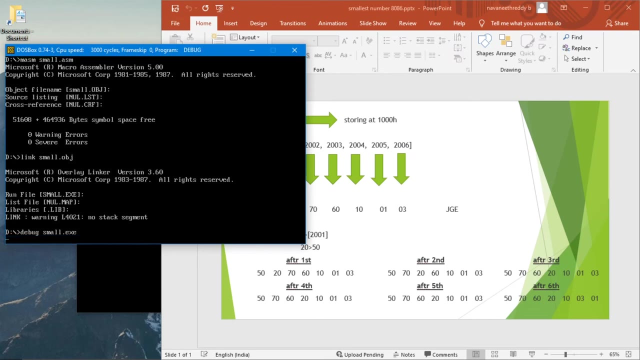 is a- don't make any mistakes over here- and click four times enter and the last command. now we are in the debugging situation, so just type in debug and just small dot exe. this time, right now. we started our debugging and the first command is: that is, we have to run our program, right? 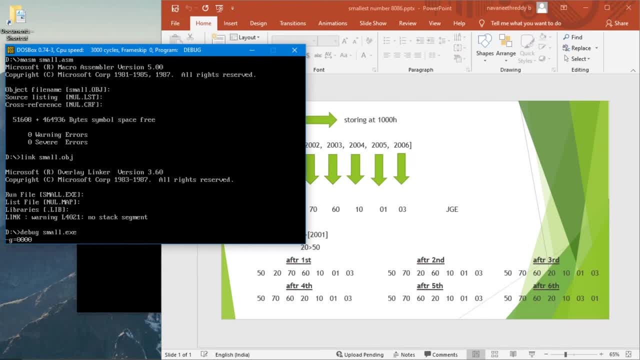 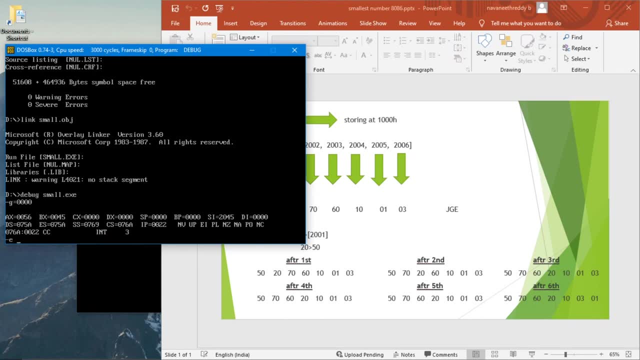 so just qg equal to zero, zero, zero, zero and click enter. now we have to provide our input values. right, we are going to give is a count value, right, the count value will be equal to the. i mean the set of numbers, that is number of numbers in our set. in our case it is seven, right, so give seven. where? 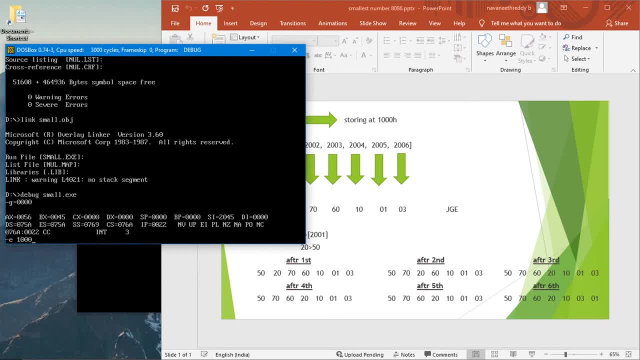 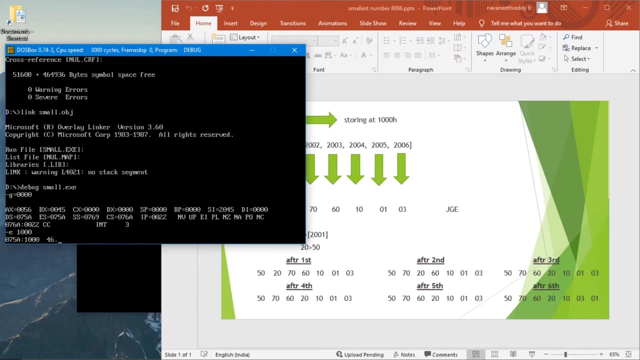 eight thousand location. that is in our case, and particularly in this program, we are giving the count value at thousand. so that's why type in e space thousand and what is the value we are going to give? that is the number of numbers in our set here. in our case there are seven numbers in our 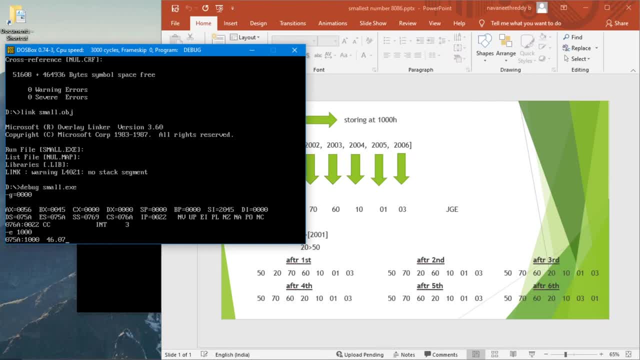 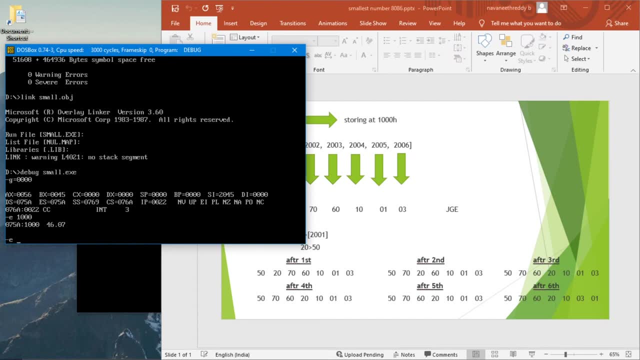 set. so just i am giving seven and click enter. now we give the count value. but what about the numbers? we have to give numbers also, right? so from where we are giving our numbers in? in this particular program 2000. so just in order to give inputs, we use e, right? so just e space 2000 and click enter. 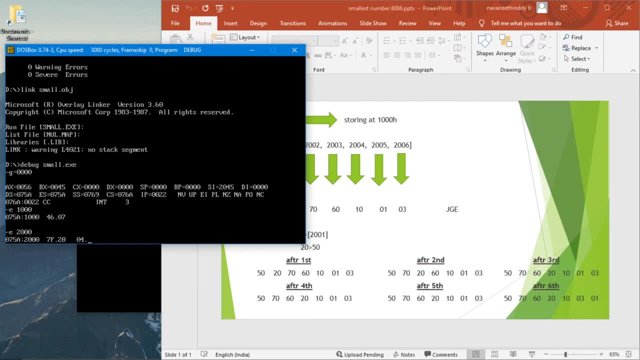 so the first value is 20, right? just a click space bar to go to next location and you can see here 0, 4. actually, what is that? 0 4 means the number which is already present at that location, that is, 2001. here, at 2001, the old value which is present is 0, 4. but we don't want that 0 4, right, we are. 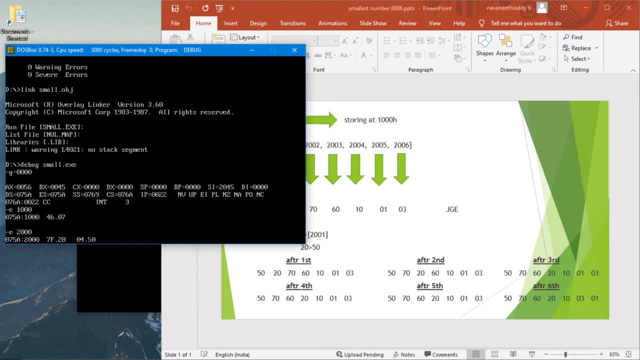 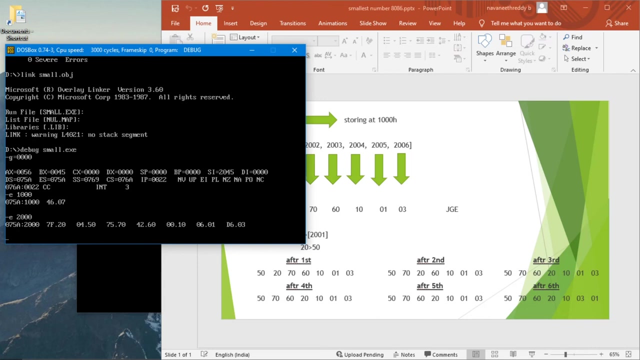 overriding. just type in 50, otherwise nothing will happen, but just. but we are not interested in 0, 4 in our case, we are giving 50. right now again click space bar. the next number is 70 space bar, 60 space bar, 10 space bar, 0, 1 space bar and 0, 3, 0, 3. now click enter. now again run our program once. 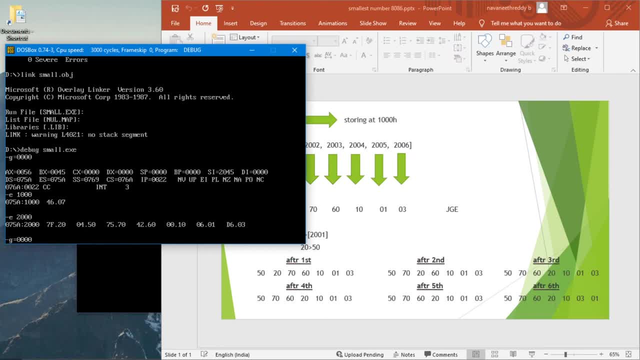 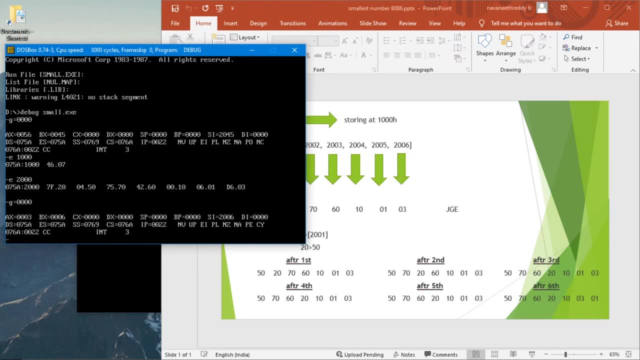 just z equal to 0, 0, 0, 0. click enter. now we have to verify our result, right, and this is a? actually we should. now, if our program runs wrong, don't be afraid we'll definitely see the mistake of what is going on actually, but, uh, we hope for the best. uh, i said that our result. 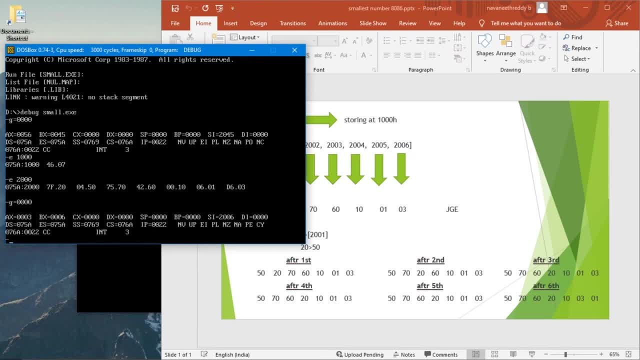 will be available in the last location right, and our last location in this case is 2006. so in order to see the result, we use d right, so just type in d space and 2006, comma, 2006. that is what the last location in our case right now, if i click enter our program should. 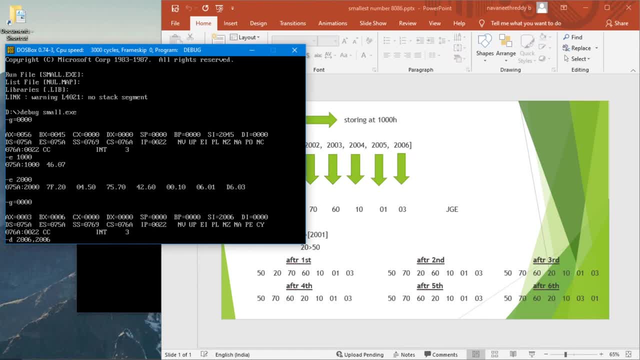 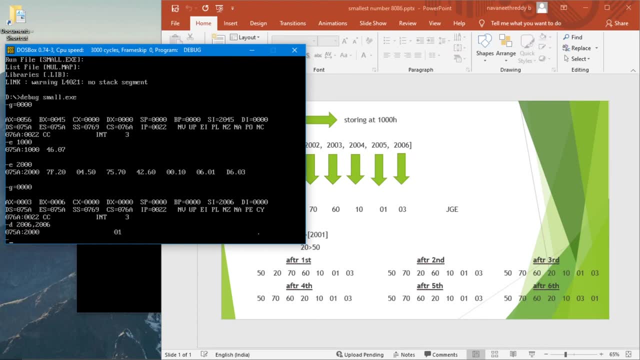 give one, and if it gives any other thing, i will be afraid. no, afraid nothing, we'll definitely figure out what is a mistake. i am clicking enter, enter, yeah, that's it guys. our program gives zero one. that means our program is working fine and fantastic. ah, i think you understood the concept.